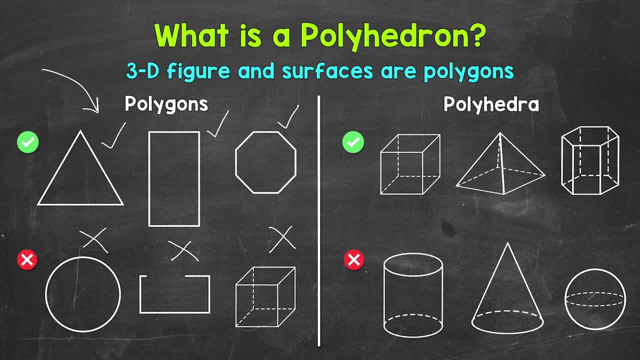 A cube is three-dimensional. Polygons have to be two-dimensional. They are plane figures, so flat A cube isn't a polygon, but it is a polyhedron. So let's move over to examples of polyhedra and that's going to help us better understand what a polyhedron is. 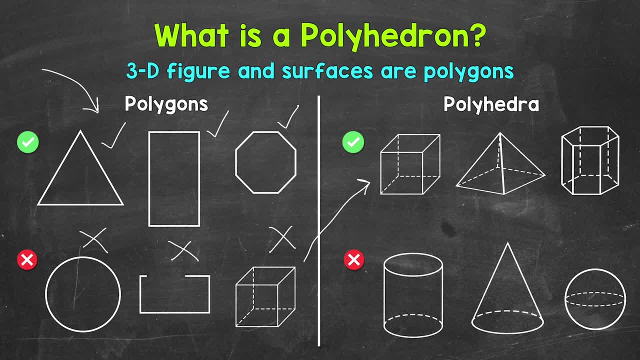 Let's start with a cube, which is a 3D figure, and then, if we look at all of the surfaces, all of the faces, those faces are all quadrilaterals, More specifically squares. So all of the surfaces or faces are polygons, So 3D, and the surfaces or faces are 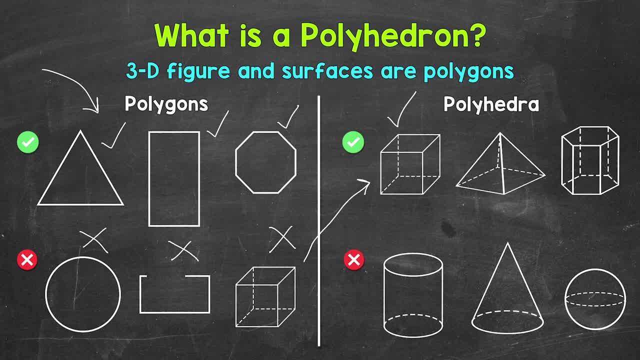 all polygons. so that is a polyhedron. Let's move to the right, to the square pyramid. That's a 3D figure and all of the faces are polygons. The base is a square, and then the rest of the faces. 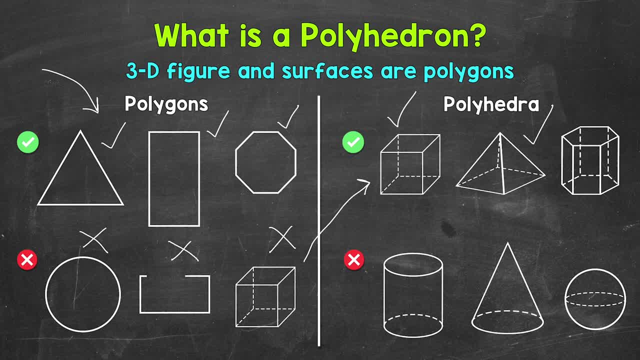 are triangles, So this is a polyhedron as well. And then, lastly, we have a hexagonal prism which is a 3D figure. And then, lastly, we have a hexagonal prism which is a 3D figure. 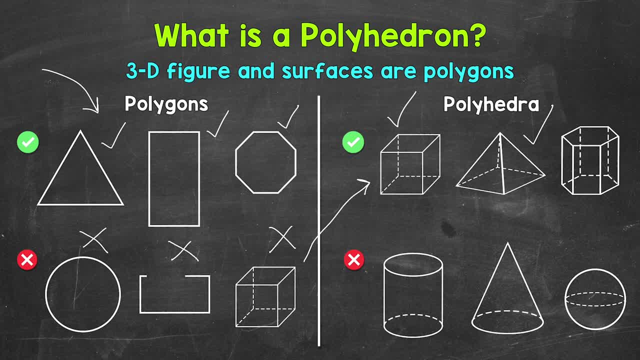 and all of the faces are polygons. Two of the faces are hexagons, and then the rest of the faces are rectangles, So this is an example of a polyhedron as well. Now let's take a look at three examples that are not polyhedra. They are all 3D figures, but the surfaces are not polygons. 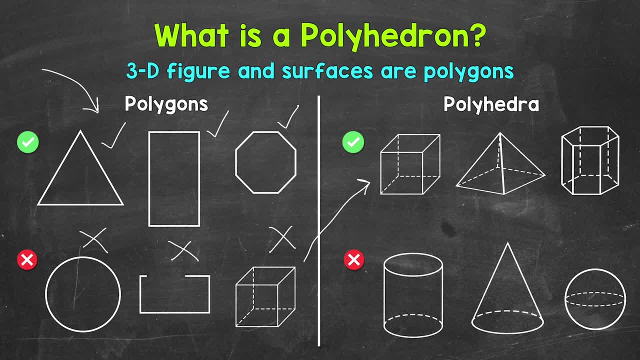 Let's start with a cube, which is a 3D figure, and then, if we look at all of the surfaces, all of the faces, those faces are all quadrilaterals, More specifically squares. So all of the surfaces or faces are polygons, So 3D, and the surfaces or faces are 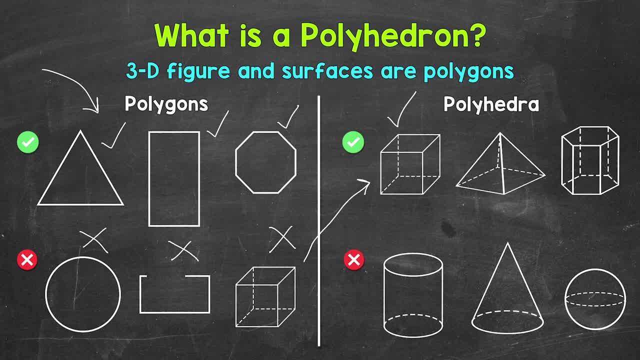 all polygons. so that is a polyhedron. Let's move to the right, to the square pyramid. That's a 3D figure and all of the faces are polygons. The base is a square, and then the rest of the faces. 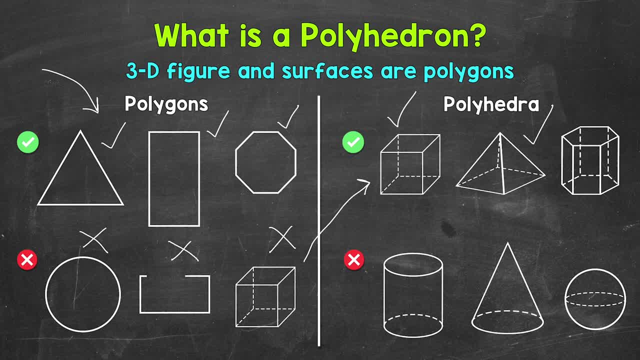 are triangles, So this is a polyhedron as well. And then, lastly, we have a hexagonal prism which is a 3D figure. And then, lastly, we have a hexagonal prism which is a 3D figure. 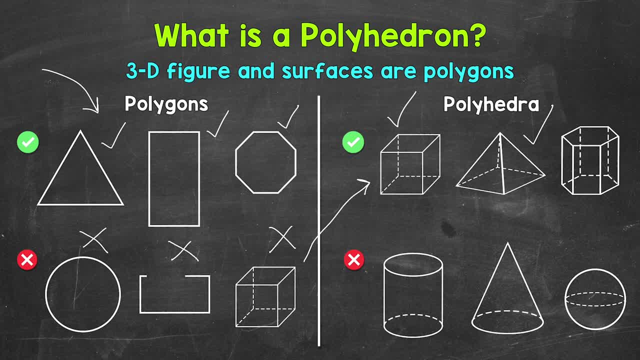 and all of the faces are polygons. Two of the faces are hexagons, and then the rest of the faces are rectangles, So this is an example of a polyhedron as well. Now let's take a look at three examples that are not polyhedra. They are all 3D figures, but the surfaces are not polygons. 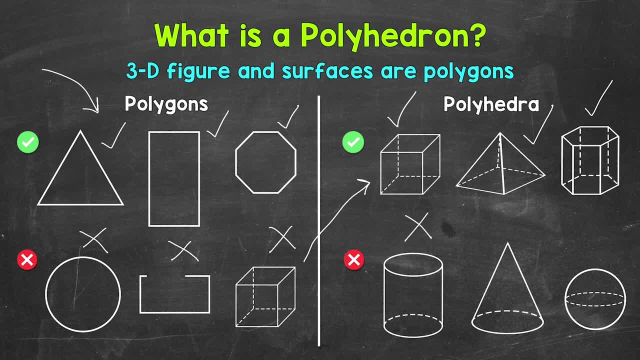 So a cylinder is not an example of a polyhedron, A cone is not an example and a sphere is not an example. So there you have it. There's a basic explanation of polyhedra. So what is a polyhedron, or what are polyhedra? Well, 3D figures and all of the surfaces or faces. 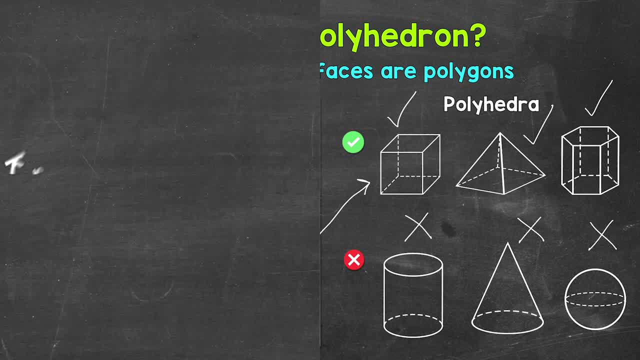 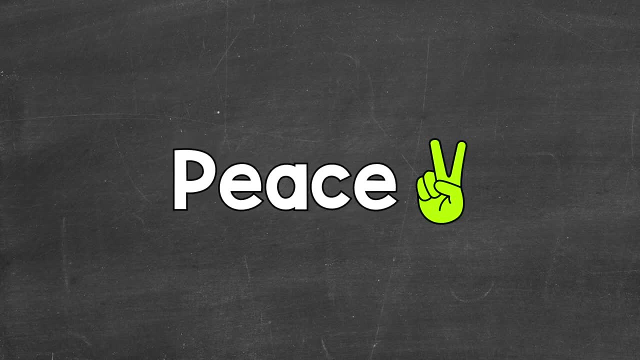 have to be polygons. I hope that helped. Thanks so much for watching. Until next time, peace Captions by GetTranscribedcom. 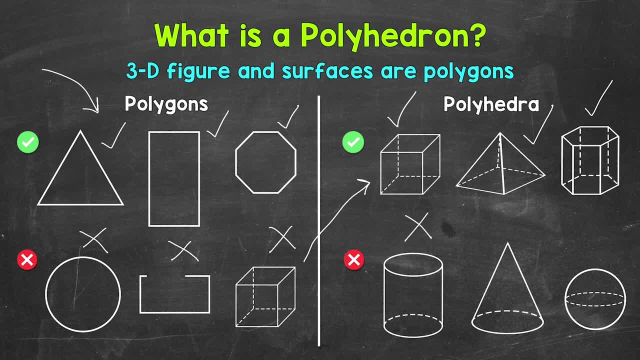 So a cylinder is not an example of a polyhedron, A cone is not an example and a sphere is not an example. So there you have it. There's a basic explanation of polyhedra. So what is a polyhedron, or what are polyhedra? Well, 3D figures and all of the surfaces or faces. 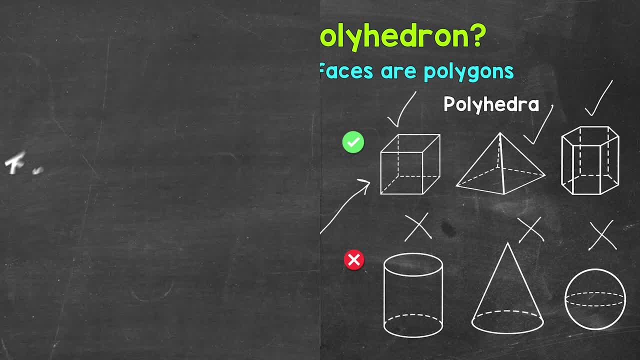 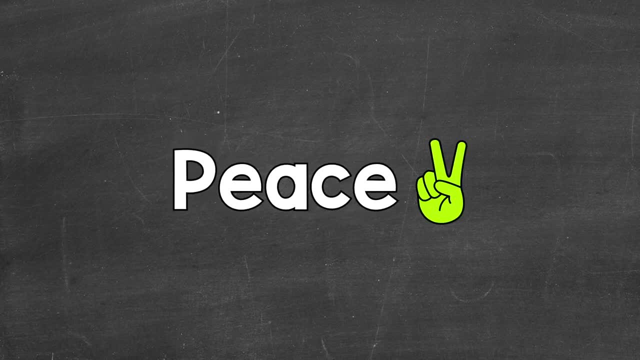 have to be polygons. I hope that helped. Thanks so much for watching. Until next time, peace. Subtitles by the Amaraorg community.